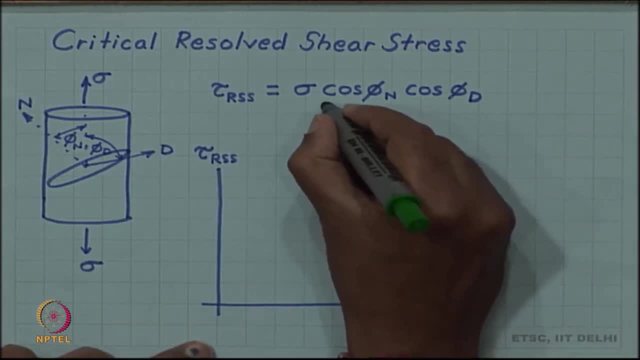 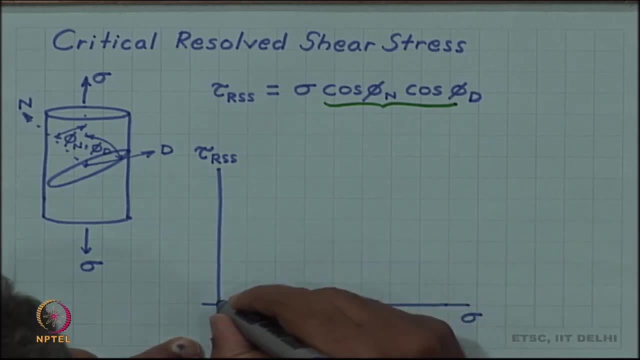 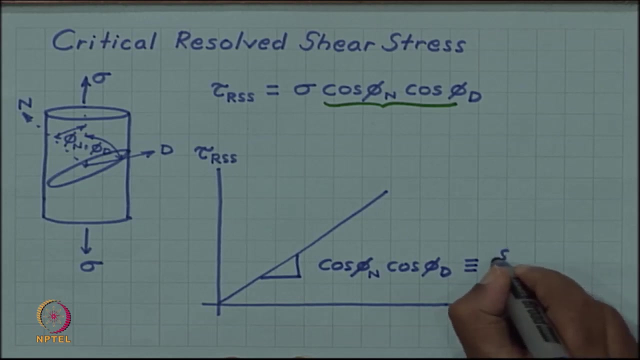 a function of sigma. we expect to get a straight line with this as our slope. So let us do that So, and the slope is expected to be cos phi n, cos phi d. Sometimes this factor is called a Schmidt factor. This product is called the. 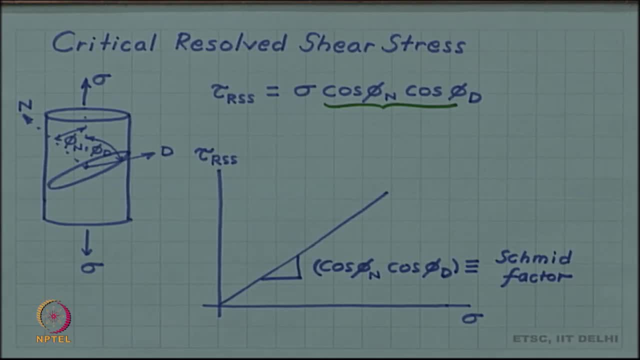 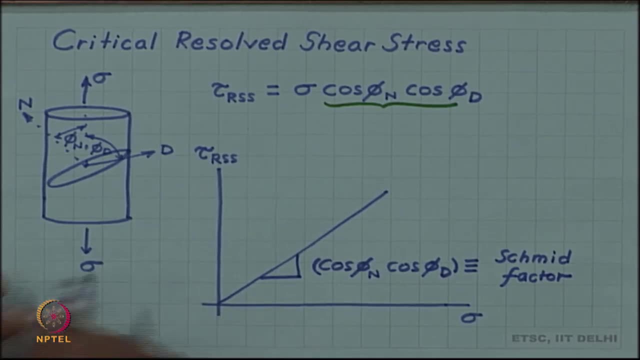 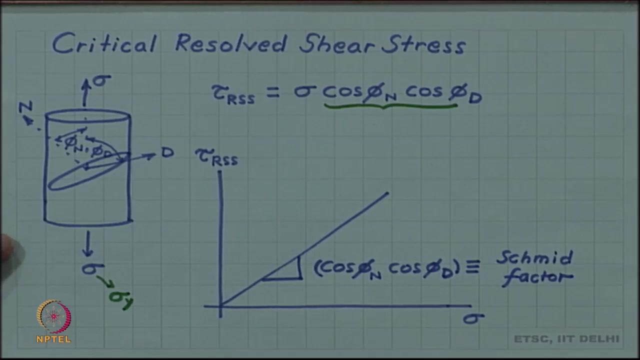 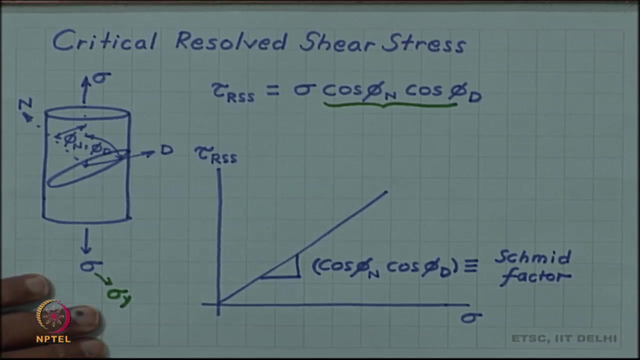 Schmidt factor. Now, if you are doing a tensile test on the sample, sooner or later this tensile stress will reach a value sigma y, the yield stress, And when you reach yield stress there will be plastic deformation. So let us now indicate that on the tensile 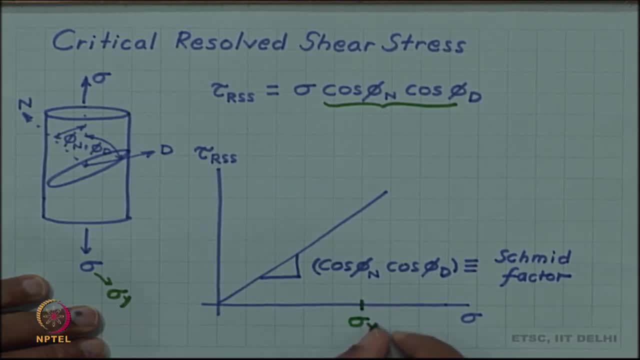 axis, there is a critical value called the yield stress, at which yielding begins. Now, corresponding to that yield stress, we can then calculate the tensile stress. Now, what we are going to do is we are going to determine the tensile stress. We can determine the tensile. 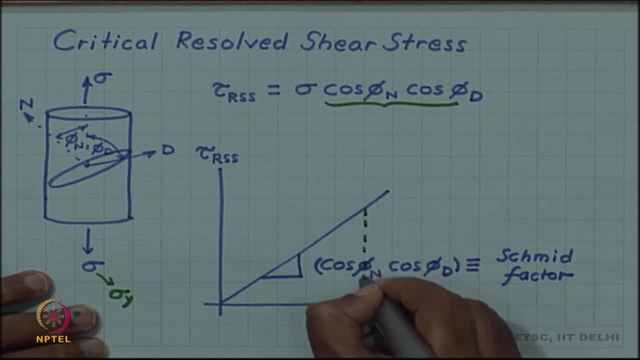 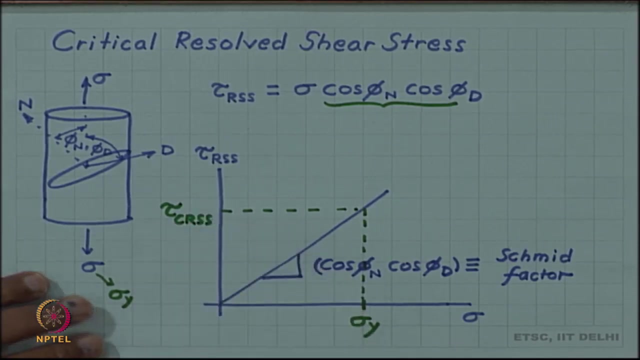 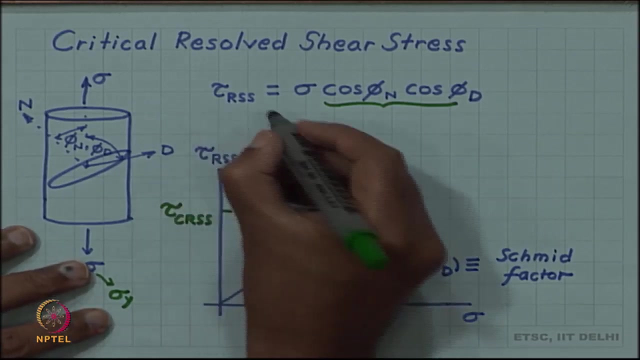 stress. we can determine the tensile stress. So in this case we are going to determine stress. if I find what is the resolved shear stress, So that value of resolved shear stress will be called critical resolved shear stress, CRSS. So which means I am increasing resolved 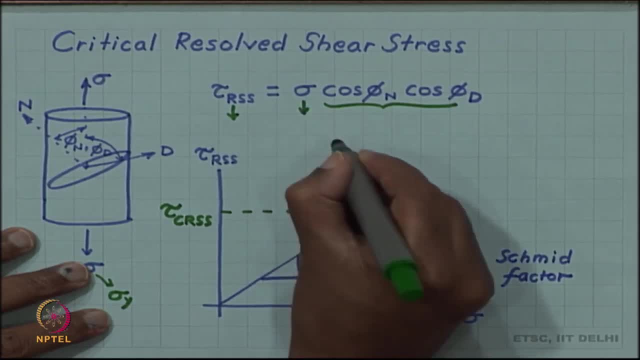 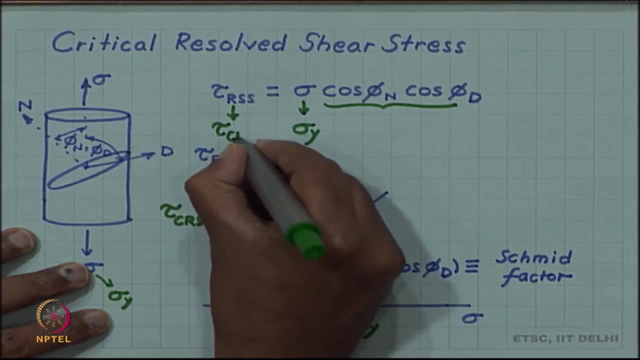 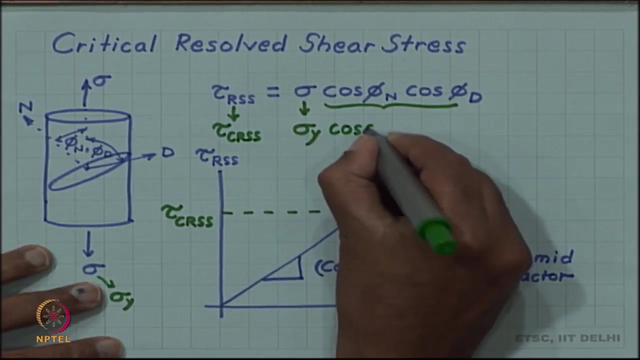 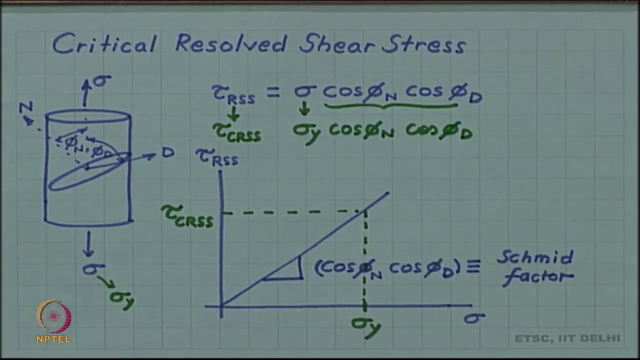 shear stress. I am increasing actually the tensile stress. Tensile stress reaches a value: sigma y. the correspondingly resolved shear stress reaches a value critical. resolved shear stress: sigma cos phi n, cos phi d. So for completeness, let us write this definition: